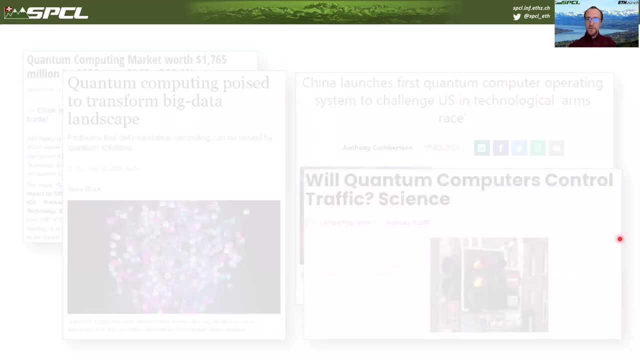 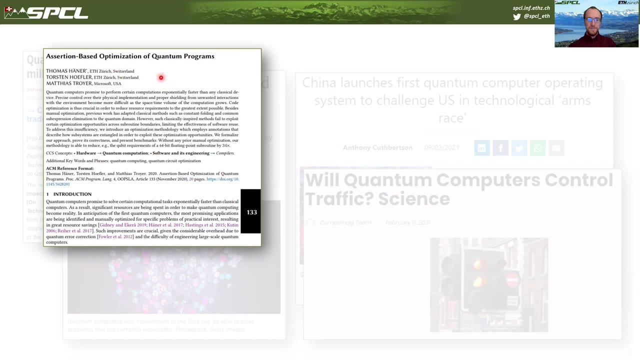 realistic, But we will see. So some of the contributions that I and my group have done to quantum computing contain, together with, in a collaboration with Microsoft, some optimization of quantum programs based on assertions, concretely Hoare logic, the first true quantum optimization, in fact, quantum compiler optimization. 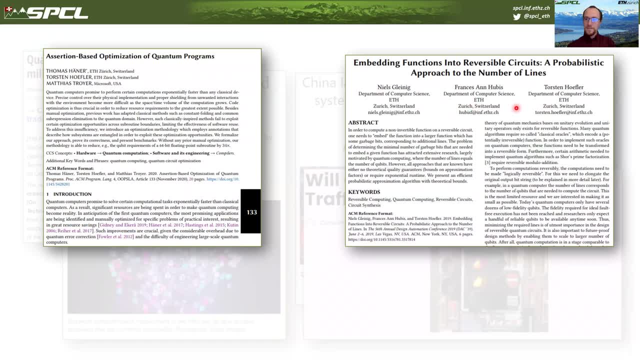 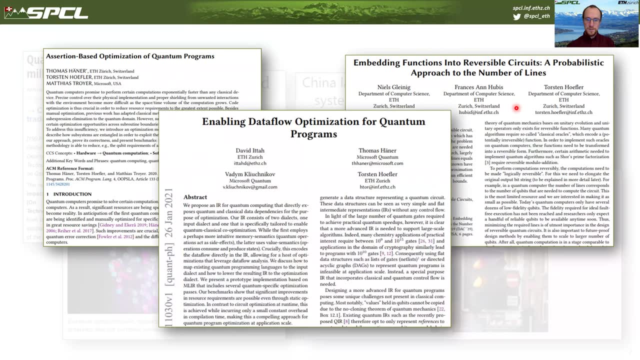 And then we have counted the number of needed lines, or ancilla qubits, in order to make functions reversible and provide a very simple lower bound proof for this. So it's quite nice, or lower bound estimate. And recently we have looked at what would the quantum internal representation actually be based on a data flow? 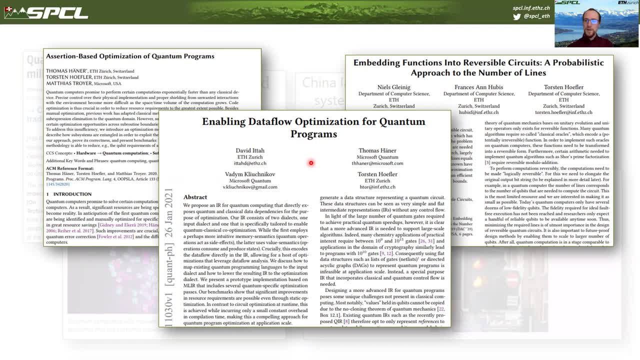 data flow models such as MLIR or LLVM in this last paper. So, but today I want to not go into too much technical depth on any of these works, because this is requiring a lot of understanding. on the side where I'm not sure if I should just give a- rather give- an- overview of quantum computing, 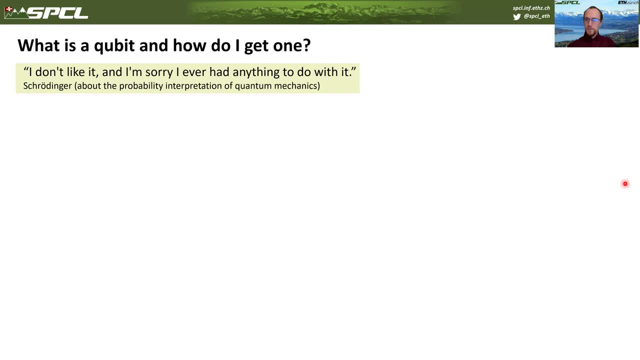 so that we can all speak the same language, and then we can dive deeper During the discussion sessions into the specifics of quantum computing or specific results. So first, what is a qubit? Well, we all know what a bit is. A bit can be zero or one. It's. 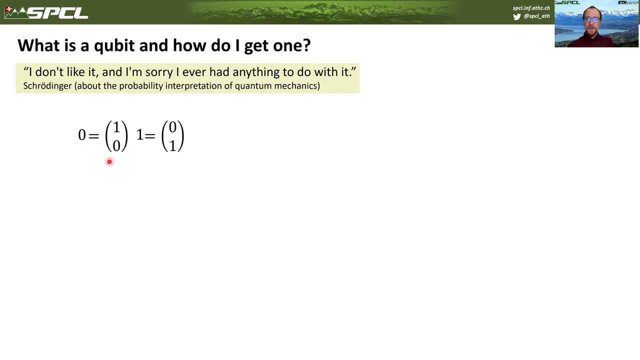 the smallest state, the smallest piece of information we have, And now we can actually write the bit as so called one-hot encoding in machine learning in a two dimensional space. So the zeros are in general, the i-th element is one, if the bit is i. So here we have only two. So we have one and two, then we can. 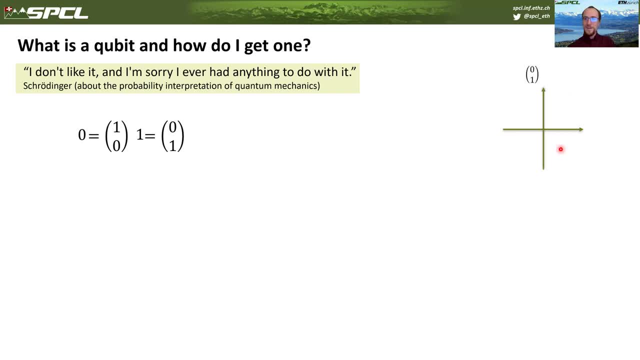 draw it in a two dimensional space. This works really well on slides. We can now draw the one in the vertical direction and the zero in the horizontal direction pointing towards east. Now I can generalize this to a quantum state, because, as we all know, quantum bits can be in the superposition kind of simultaneously in the zero and one state. 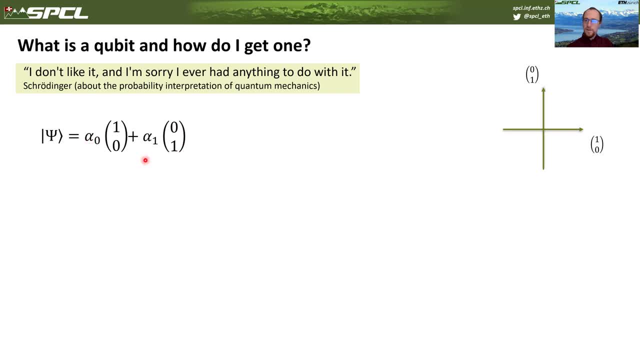 And the intensity or the probability when I observe one of those qubits in either zero or one, is reflected in the so called amplitude, which in this case is alpha 0 for zero and alpha 1 for one. and these amplitudes square are actually probabilities, which means that all the amplitudes square summed up equal one. 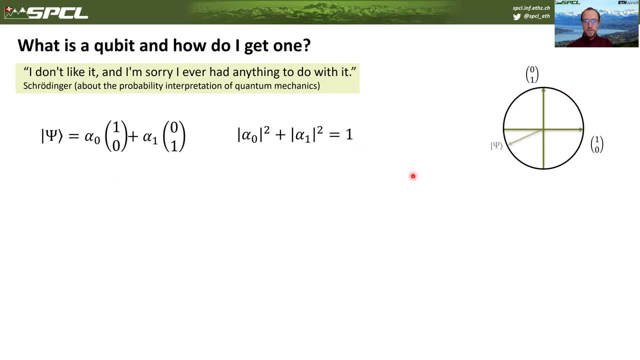 And this in this two-dimensional visualization forms the unit circle. So now a quantum state like this psi here could for example be here, if both of them are negative, the alphas. So then I can rename these states to be more convenient in the so called braquete notation. in this case it's a ket here. 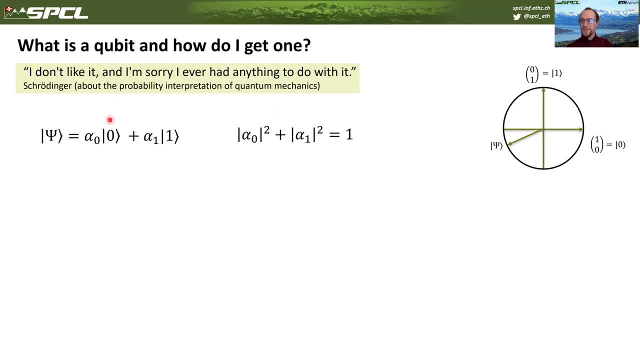 with zero and one, so that we don't have to write very long vectors, because these vectors will be of size two to the n for n for a quantum system with n bits. and then this is the very famous plus state, which is really where the qubit is absolutely. 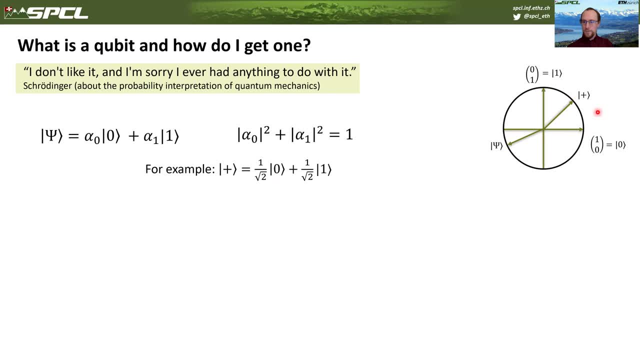 undecided between zero and one. so it's a 50: 50 chance to go into either of those states. when measured, this is great. um, so now you can argue, or i could argue, that we can actually encode a lot of information in these alpha zeros, in these amplitudes and alpha ones here, um, unfortunately, 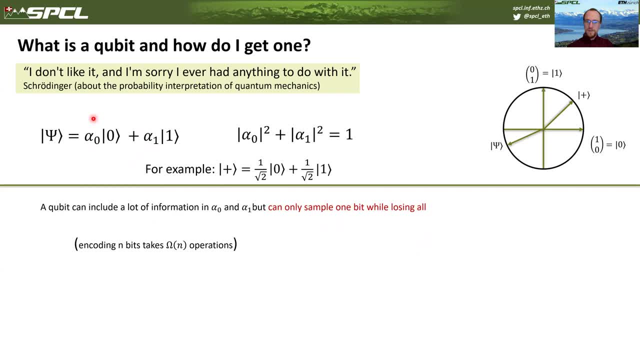 i can only extract one bit out of a single quantum bit when i measure it, so that we can encode a lot of information. but we cannot really measure a lot of information. so we can exactly measure from an n-bit quantum system. we can measure n bits because there is a very restricted. 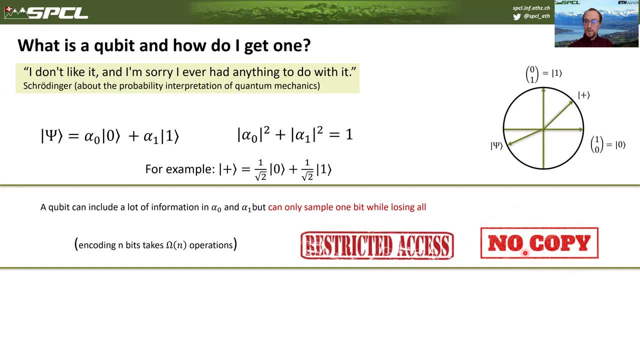 access function to this quantum state, and i cannot copy a quantum state. if you could copy it, then you can simply sample it and get the probability distribution um reverse engineered, so to say. but unfortunately we can also not copy it um. so however, it's still pretty powerful. 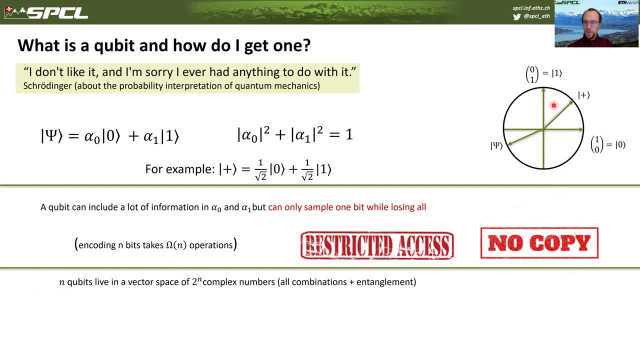 because n qubits live in a vector space of two to the n. with this formulation that i discussed here right, and we can write this shortly- as the sum of these alpha i's and then each of these states from going from 0 to 2 to the n minus 1. so for 2 bits, the possible combinations, as we all know: 0, 0. 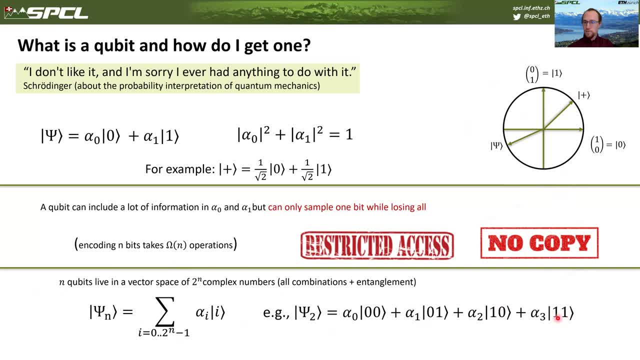 0, 1, 1, 0 and 1: 1, and then we have four different, so two to the n, two to the two, in this case um, four different alphas that encode the probability distribution. alpha is, by the way, a complex number in general quantum computation. 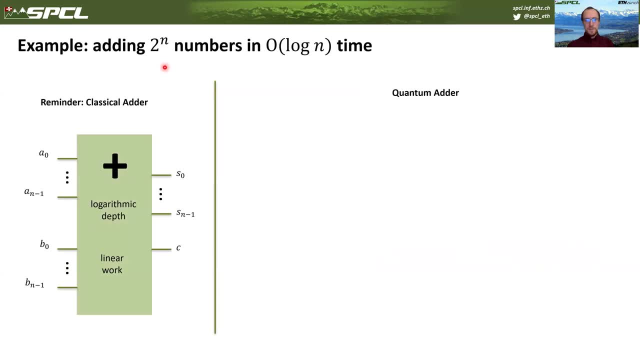 so, not, so, not not. I can demonstrate you how to actually implement an adder circuit that adds two to the n numbers in log n time. So you all know a classical adder which takes two numbers, two n-bit numbers, a and b, and outputs a sum and a carry bit, And it does this in logarithmic depth and linear arc. 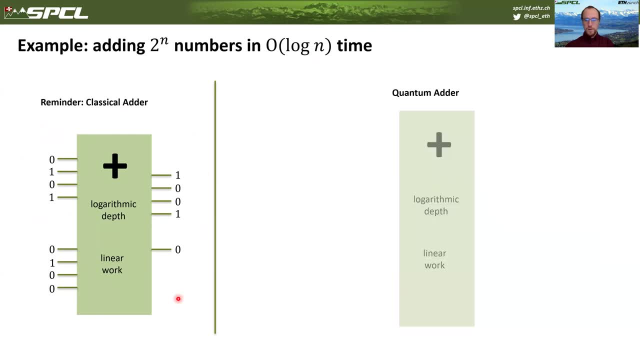 So we can feed in specific numbers here and get a specific output: A quantum adder. just believe me, we can do the same thing. We can implement an adder with logarithmic depth and linear arc. We have part of the quantum state, the number a, an n-bit number, and part of the quantum state. 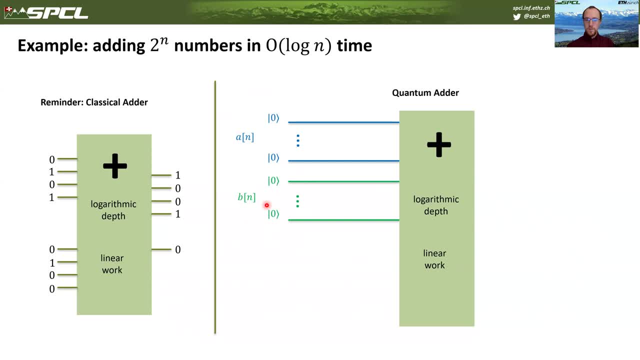 a number b, The initial quantum state is almost always for a quantum algorithm, zero. And then we have a set of additional bits that we call ancilla or garbage bits or additional helper bits that I don't want to talk about, But this is exactly the second paper that 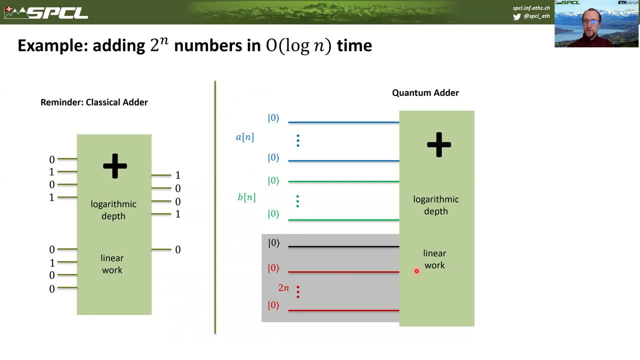 I mentioned in my introduction that we've been working on to assess for a given function, like this adder, for example, what is the minimum number of needed bits to ensure reversal. So we can do this in the quantum state And this is the first function in the quantum state. 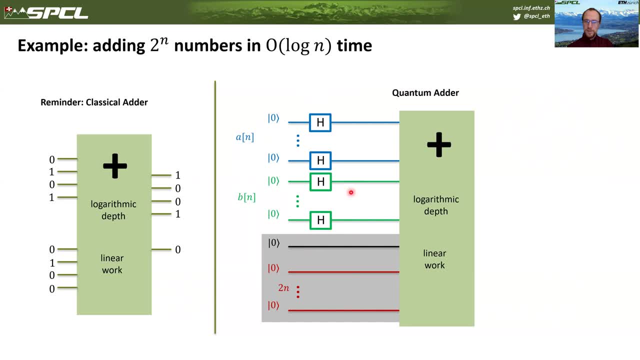 which is the set of Hadamard gates, which puts the quantum state from the all-zero state in the completely undecided state. So basically, any bit pattern is equally likely in this completely undecided Hadamard transformed state. So then we have the final state after the adder, which is: 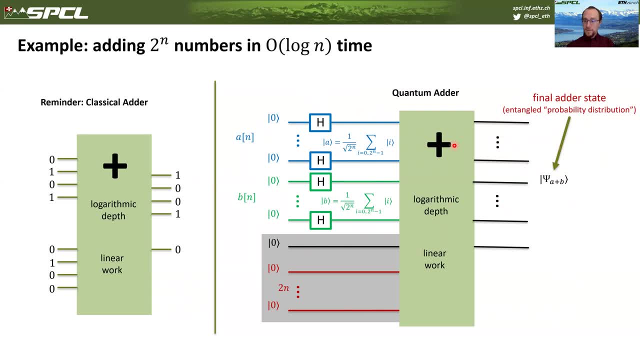 really the sum of the two. So it's the sum of the two. So it's the sum of the two that we're talking about here, And then we have the final state, which is the sum of the two. So it's the. 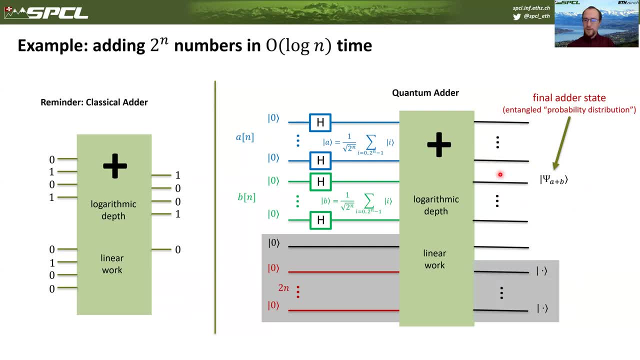 sum of the two that we're talking about here, And then we have the final state, which is the sum of the two that we're talking about here, And then we have the final state, which is the A itself is on the top bits, But then A plus B is on the remaining bits, And then we have 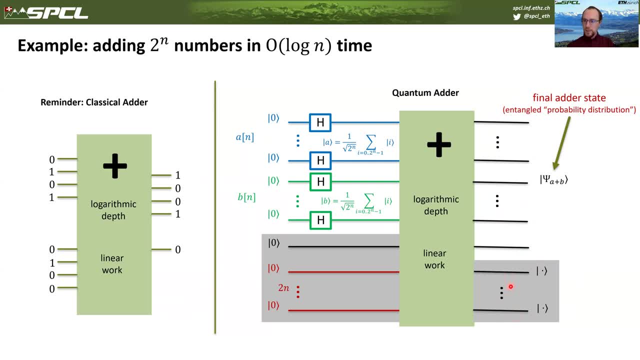 additional garbage bits which we don't really care about what they do, But we need them to express the problem in a quantum mechanical formulation. So here's an example with two two-bit numbers. So here you see the input state to the adder And then the output state is. 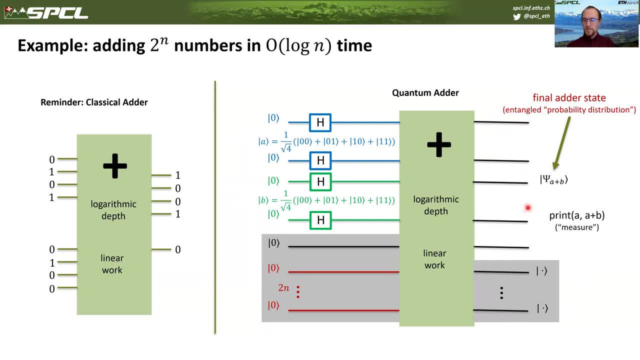 of course A on the first n bits and A plus B in the second n bits, And then there's a carry bit as well. But now the question is: how do we get to this state? Well, the only way to get to this: 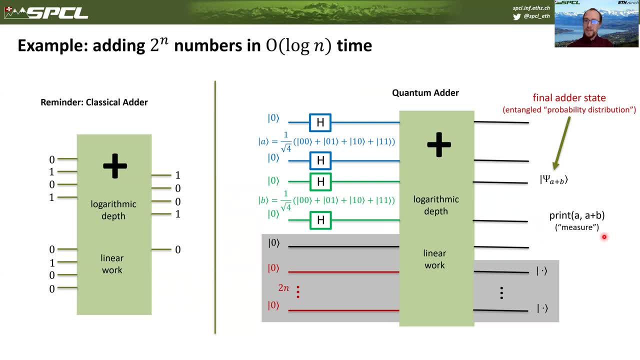 state is to actually measure it, to transform it into the classical world where we live in, where we can observe the state. We can print it on a specific device And we can look at it, But as soon as we do this, we will actually destroy the quantum state And we will get one. 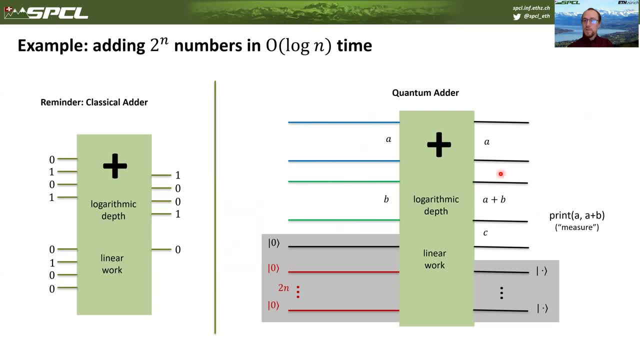 particular choice for A and B as the inputs And then of course the correct A and the A plus B and C as the outputs. But we cannot choose that choice. So basically, it's an arbitrary bit pattern that we get as an input And of course the correct A plus B as an output. But it could. 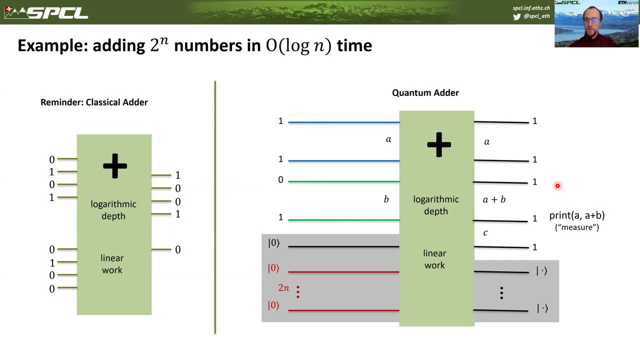 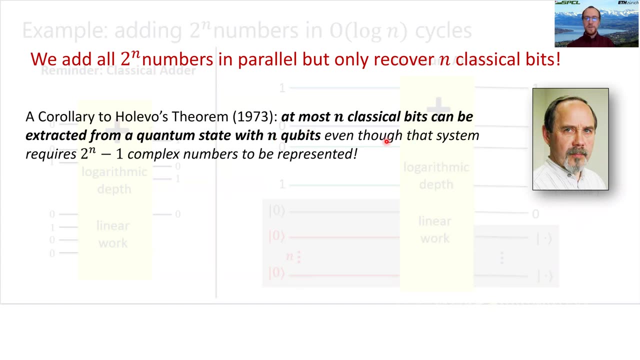 be this, It could be this, It could be any bit pattern, And we have absolutely no influence on this for this particular construction. So that's not such a useful adder. In fact that somewhat generalizes to using Halevo's theorem that essentially, at most n classical bits can be extracted from a quantum. 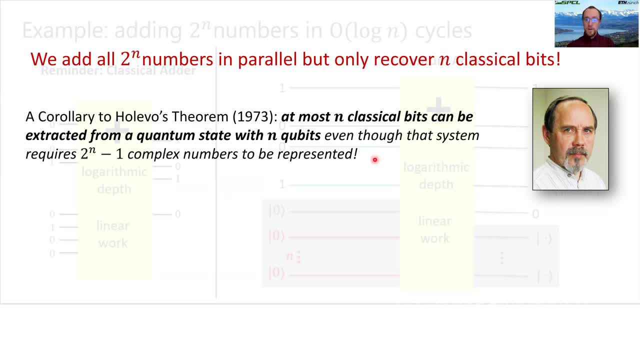 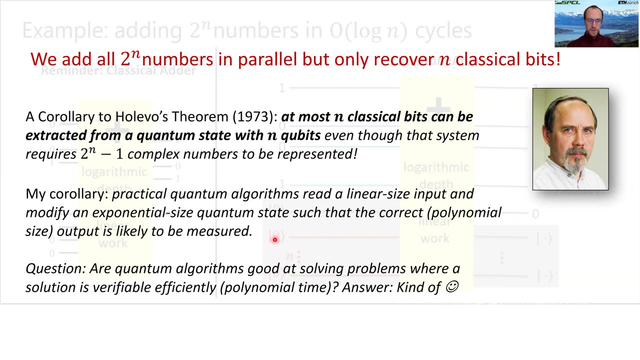 state with n qubits. This is what we are doing, even though that specific quantum system requires 2 to the n minus 1 complex number, so at least bits to be represented, OK. So that's unfortunate, And actually my personal view on this. we could have a corollary to this corollary. 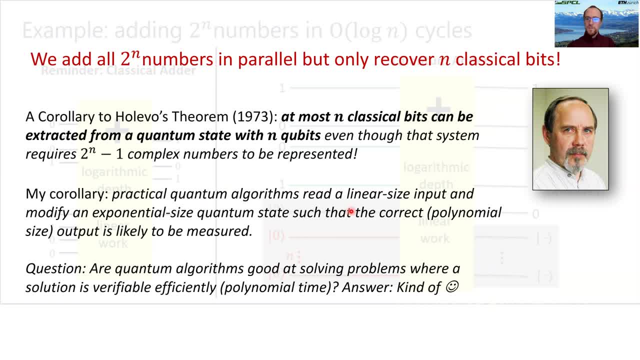 is that the practical quantum algorithm must read a small input in brackets linear size and modify a very large in brackets exponential size quantum state. so to get a speed up- because these quantum queries are relatively slow compared to classical computers- that the correct polynomial size output in brackets is likely to be measured. So very 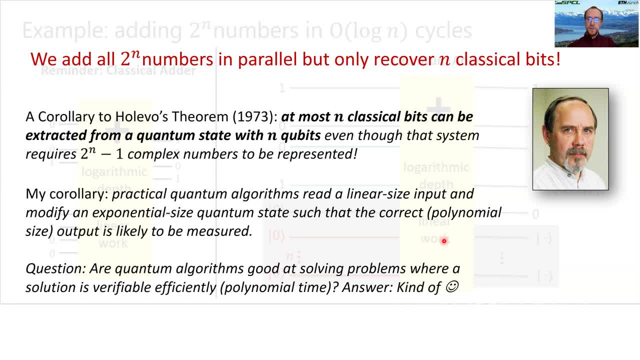 small input, very large search space that we are searching with this quantum computing device, And then relatively small output again, because we will need n operations to encode the input and the output. we can only measure once and we get our result, And this is also only n operations. 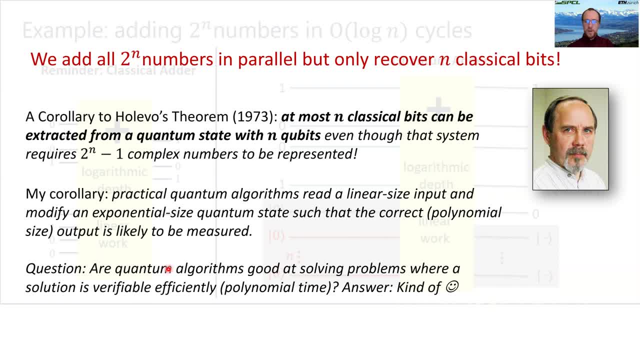 if you have n qubits. So really what this means. quantum algorithms are good at solving problems where the solution is verifiable efficiently in polynomial time. Is this true? Well, we are probably reminded of a class of algorithms that are NP-complete problems. 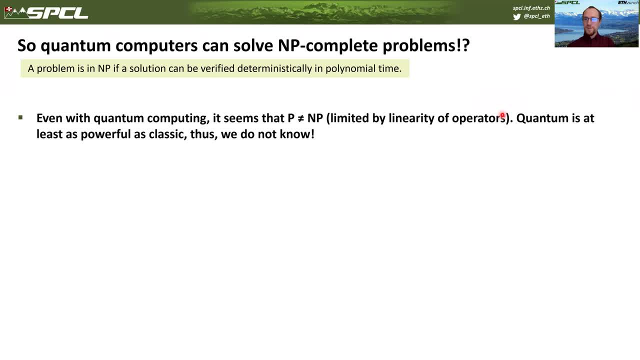 where I was very excited to join the quantum team and I thought we would be solving many of those. Of course I was proven wrong, not so fast. It seems that P unequals NP, even for quantum computers limited by the linearity of these operators. Of course we can tell for sure, because we don't. 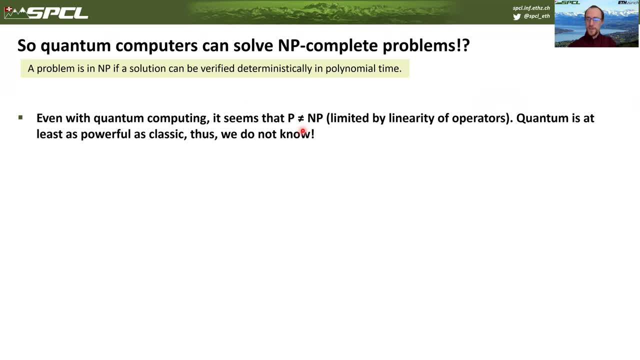 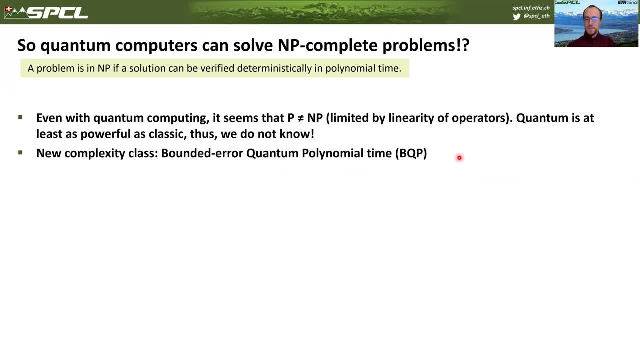 Quantum algorithms are probabilistic algorithms, So you sample them with the very high probability to give you a correct result And, as we just mentioned, this result is almost always easily verifiable whether it's correct or not. And this is strictly more powerful than the bounded error probabilistic polynomial time. 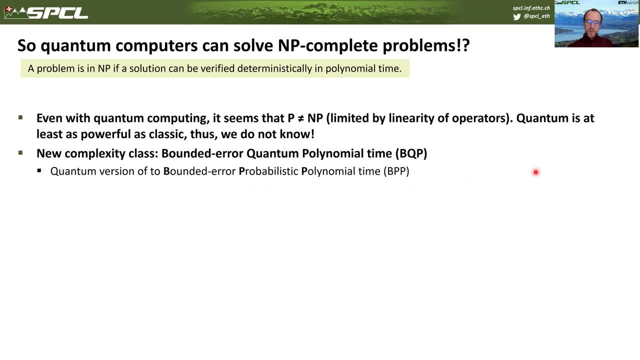 algorithm. So probabilistic algorithms are pretty powerful, but quantum algorithms are even more powerful because you can have negative amplitudes. So two amplitudes added together could actually get the result of zero, which is impossible for probabilistic computers. So that's the main. 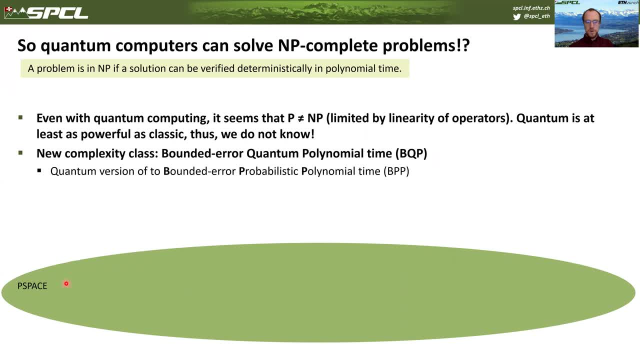 part of the power of quantum algorithms here in this thinking model. So if you now draw the number of algorithms solvable in polynomial space, you of course know that the non-deterministic polynomial solvable algorithms, so the ones that can be checked in polynomial time or verified, 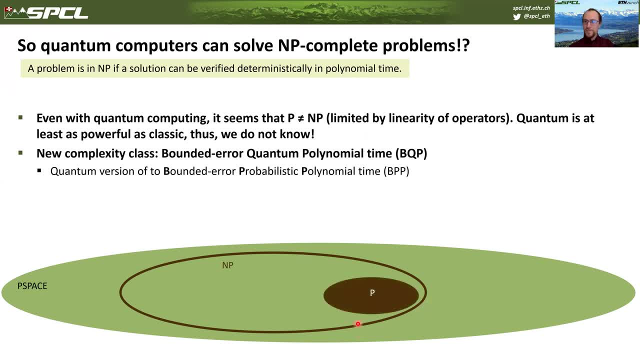 is a subset of those. We also know that the ones that can be constructed in polynomial time is, of course, a subset of those. We also know that the NP-complete problems is a subset of the NP-class problems. We do not know whether NP equals the NP-complete class, equals the P class in classical, as. 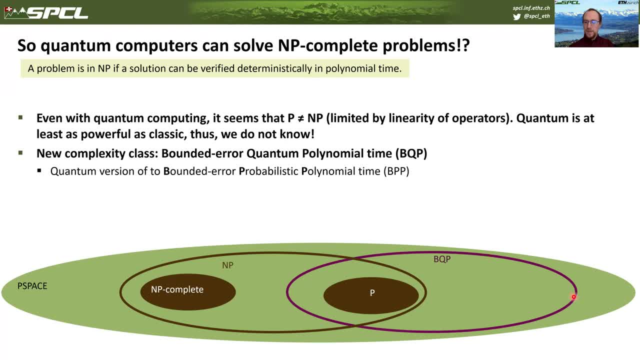 well as in quantum, of course. But we do know that the BQP set of algorithms, so the algorithms that are solvable on a quantum computer in polynomial time with a bounded error, is larger than P and is also larger than the ones that can be solved with a probabilistic polynomial time algorithm. 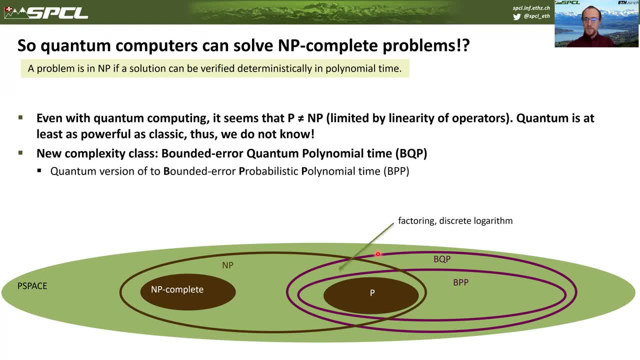 where we basically assume a random number generator. So the examples that we know that we can construct is factoring in discrete logarithm algorithms which, based on quantum Fourier, transform. So it's another interesting set of algorithms which is drawing from the NP-intermediate class. 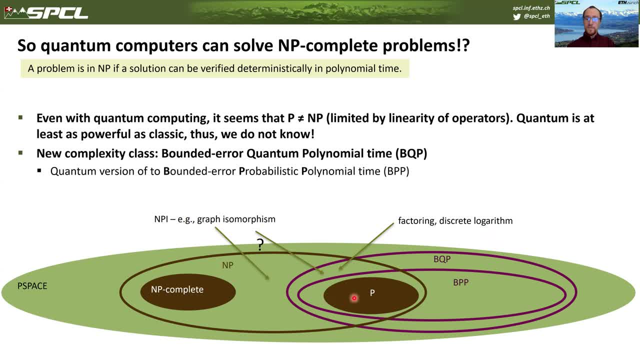 So these are not NP-complete or not known to be NP-complete, and these are also not known to be solvable in polynomial time. so we don't really know where they belong And it's not clear if those like graph isomorphism, for example, 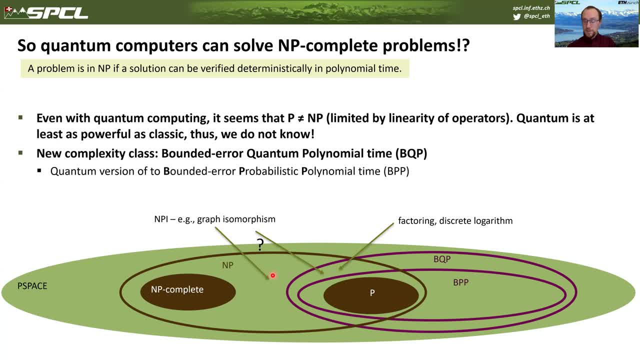 is actually solvable on a quantum computer or not. So there are lots of interesting open problems for theory researchers on the algorithm side in the quantum computing area. But, as I mentioned, I'm a systems researcher and most of us are probably systems researchers. So how do we build? 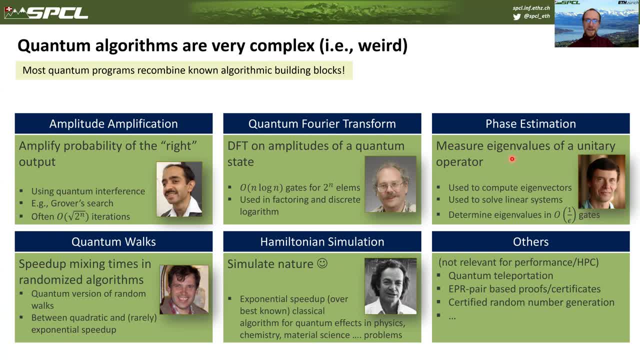 real quantum algorithms. how do we write a quantum code? And unfortunately, to my surprise, quantum algorithms are extremely complex and somehow weird. It takes some time to get used to it, At least for me, what these algorithms do And in fact most of the algorithms I've seen, most of the programs they base on a very small number of. 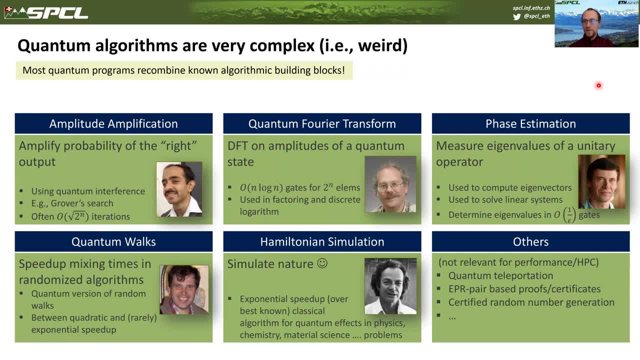 fundamental algorithms. Many of these fundamental algorithms, or building blocks I would call them, is actually based, even named, on the inventor, and only every decade or so. there are at most two of these algorithms invented. So, for example, Grover's algorithms, or sorry, Grover's algorithm, or Shor's. 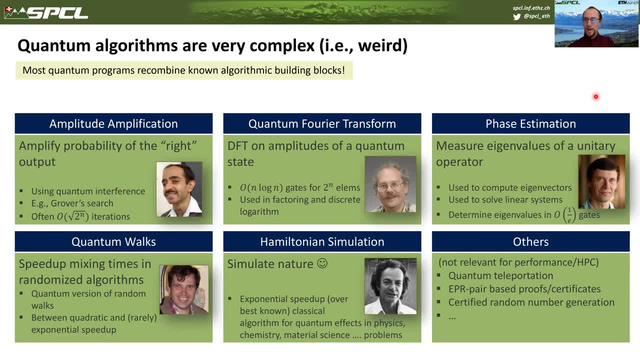 algorithm and so on. So there's only a handful, maybe two handful, of these basic building blocks and we derive everything else from those, because it is so hard to come up with a good quantum algorithm. And to give you a little bit of an intuition, I want to show you one quick example. 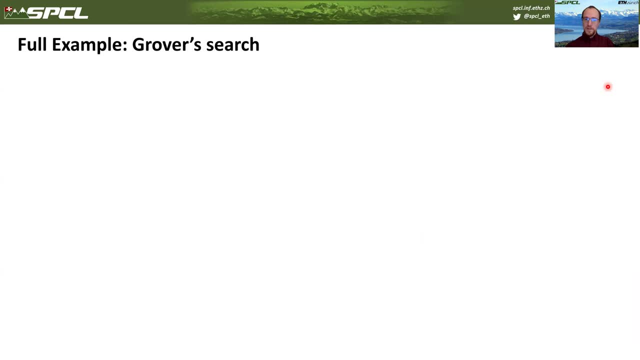 of one specific algorithm, Grover's search, which in my opinion is the simplest, somewhat useful algorithm. We will see. it's not really too useful, unfortunately, but it's still the simplest that I can explain in a single slide in a couple of minutes. The idea of Grover's search is that 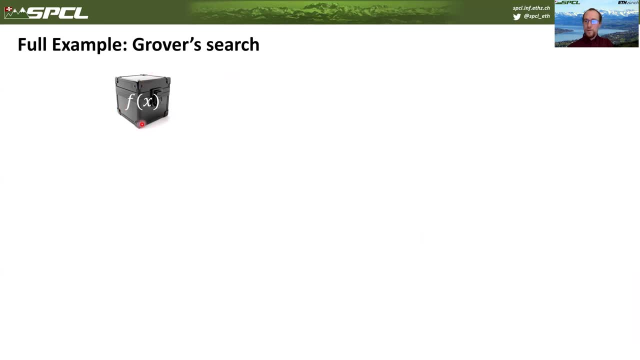 we have a black box function f of x which we are not allowed to look at the structure of the function, but we can evaluate it. So the function accepts certain inputs from a domain d and produces certain outputs in the in an image c. So the set of valid inputs is d, the set of valid 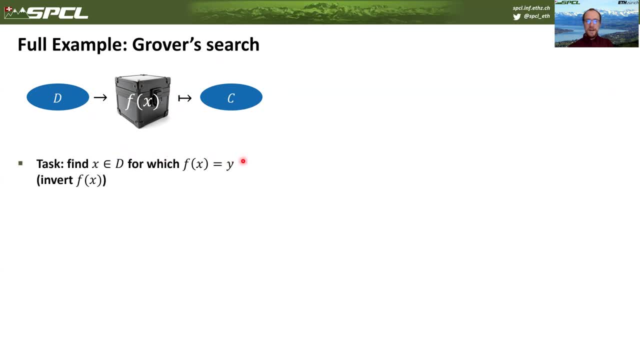 outputs is c. So now I get the task. I have a function invocation for some variable, x that is evaluated to y, and I want to know x. and let's assume this function is bijective, just for simplicity. So really, what I want to do is I want to invert f of x, but of course I can't really look. 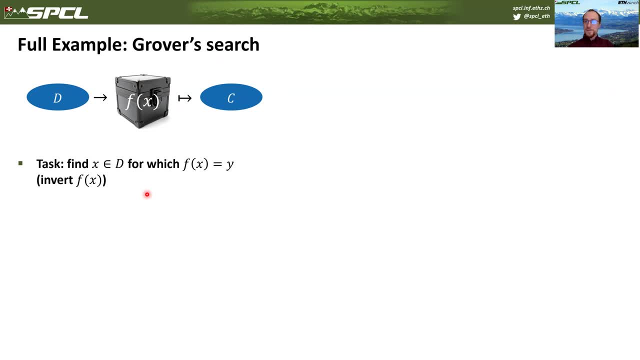 at it. So f of x may be d doing anything. but I'm not allowed to check, I can just invoke it, which means classically I need the problem with high probability sampling at least the cardinality of D half queries. 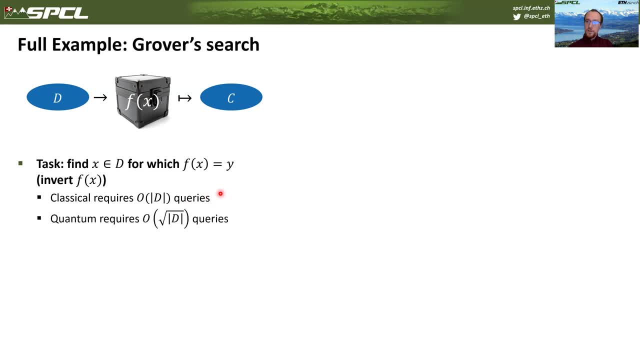 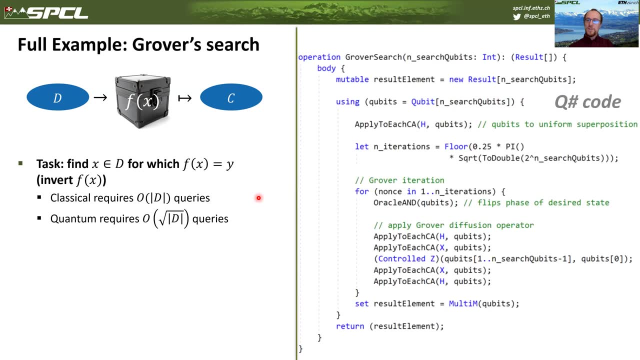 or O of D queries in the classical computing world. Interestingly, in the quantum computing world I can do this with square root of D, of the size of D, which is quite cool. And let me show the algorithm because it's quite simple in Qsharp. 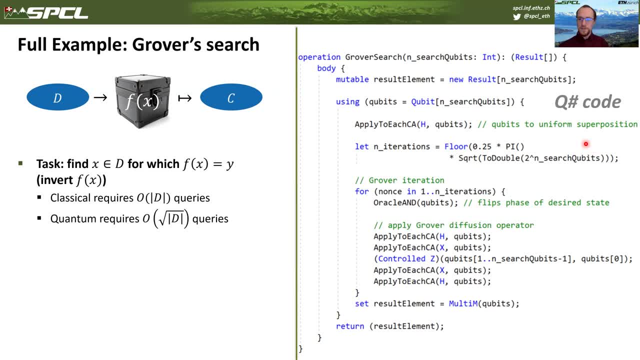 That's the Microsoft quantum language, which I highly recommend looking at. It's a very highly productive language. I wrote this example code in a couple of hours and I can even explain it to you in a couple of minutes. So what we first do here. 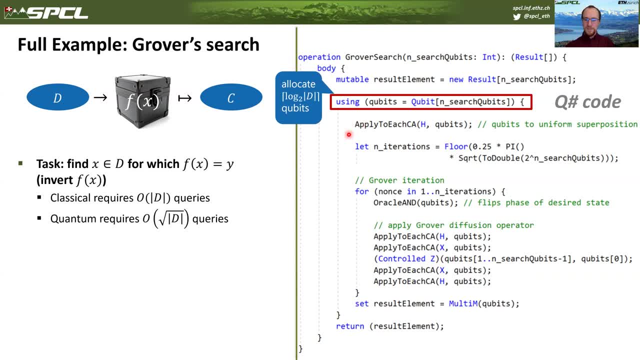 it looks like normal C code, in some sense well inspired by Fsharp, but it's like normal imperative code. What we first do is we allocate logarithm of the size of our domain, many qubits, because that's what we were going to feed in. 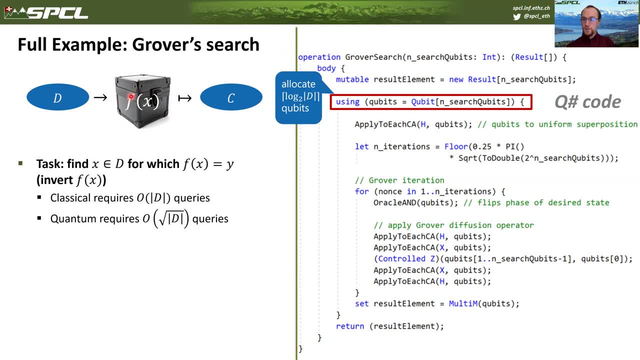 Remember, we're going to work on a superposition of all possible inputs to this function at the same time, So we need log in many of those bits. These bits are initially all zero, So going from zero, zero, zero to one one one. 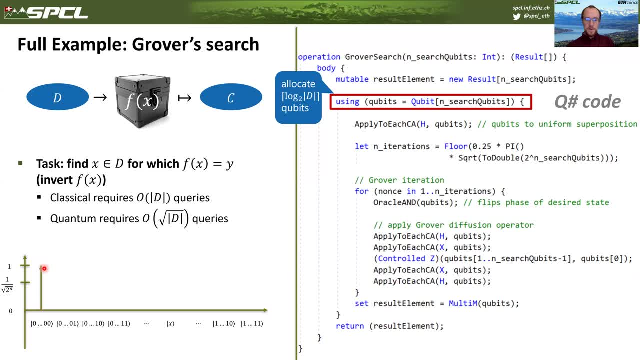 But, of course, all these bits. so the probability distribution, as we were seeing here, for all of them being zero, is one and everything else is zero. Well, the first thing we do in most quantum programs that I've seen is we apply these Hadamard gates. 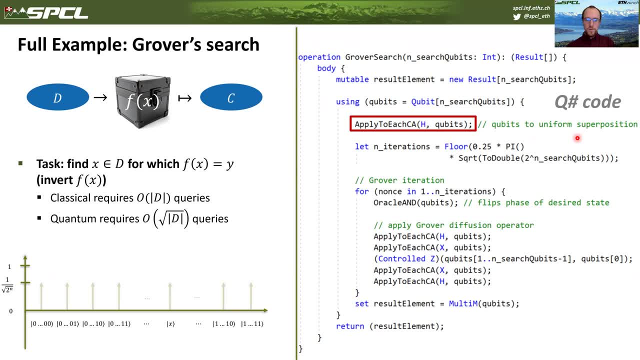 to each of the qubits individually, which means we transform them into a so-called uniform superposition that any bit pattern is equally likely. now So, and the likelihood of each is of course one divided by square root of two to the n. 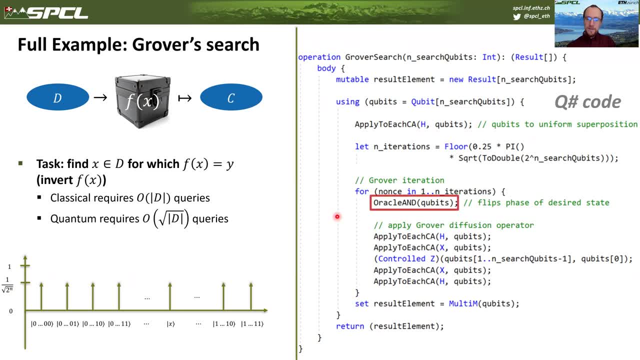 Well, that's the amplitude and the square of this is the likelihood Moving into the so-called Grover iteration. and then there's one trick that you just have to believe me, it's not too hard, but I don't have time to explain it. 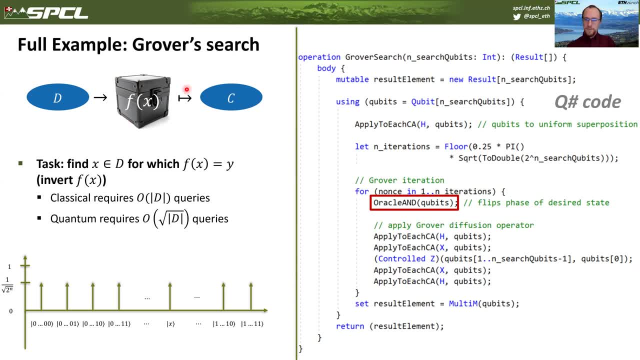 is, you can implement an oracle of this f of x function in quantum computing, in a quantum computer that will flip the amplitude of the correct y output. okay, So by flipping it just negates it. And then there is a second operator. 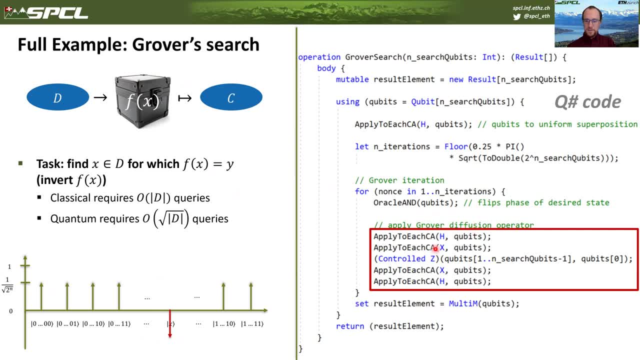 that's called the Grover diffusion operator, which what it does- it's also relatively simple to explain. It reflects each of these amplitudes at the average of all of the amplitudes. So this is now the average, because we flipped one. 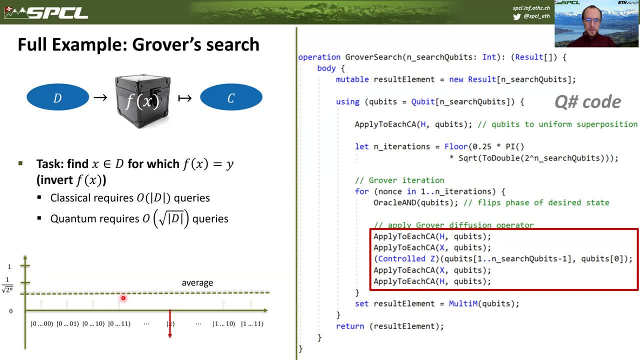 of course it's below the original average And now we reflect on this average. So those will all go down proportionally and this, the bottom, will go up proportionally. So now we keep doing this, We apply the oracle, which will again negate the correct output. 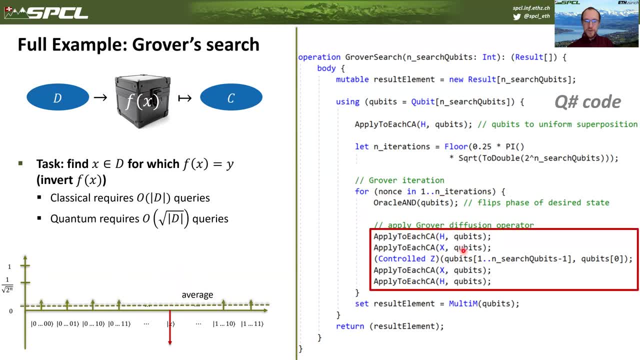 And we apply this diffusion operator again. Now we can see why it's called diffusion operator, because it really diffuses all of the not relevant input states down to close to zero. And if we keep doing this square root n times, we will have a very high probability. 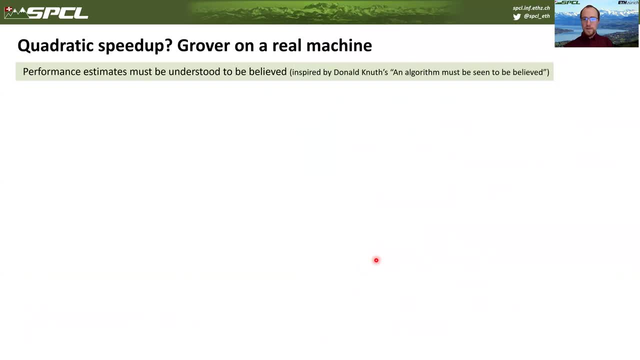 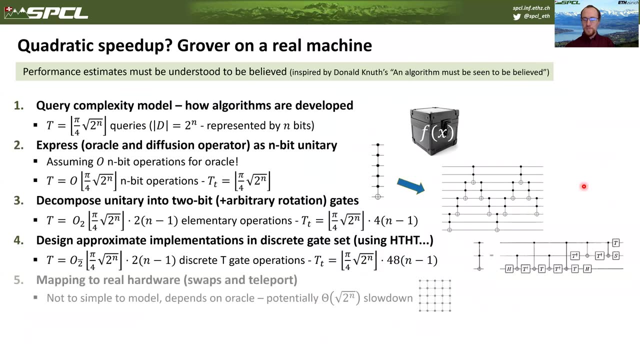 of observing the correct output state. Right, this is Grover's algorithm, and then we are done. So now the question is: well, is this as simple as I explained it? Of course it's not, because you need to map this to a real machine. 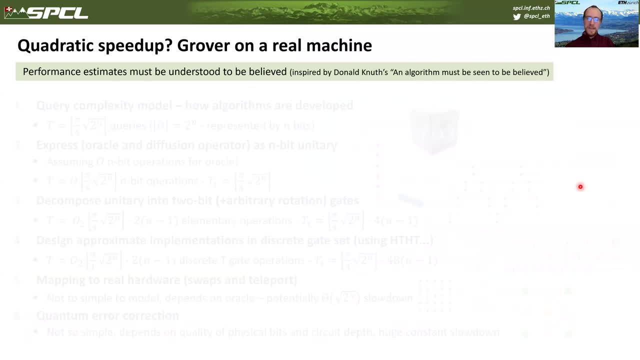 all these systems aspects and all the quantum error correction and whatnot, And actually if you wanted to, let's say, invert the AES function so an encryption function, you will in practice not go much further than about 50 and maybe 60 bits today. 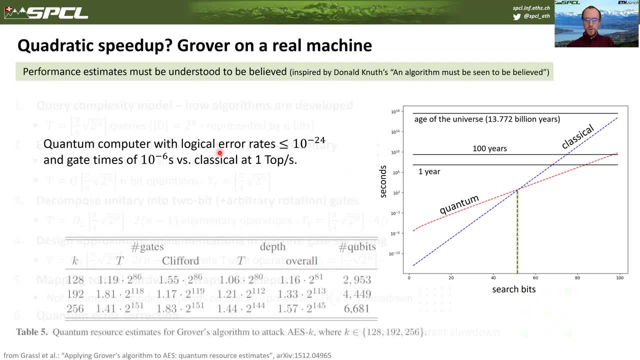 So that is not satisfactory, given the reasonable quantum computer. In fact, if you want to crack the real AES algorithms- colleagues have done a study on this- it would still take a very, very long time. So AES is secure for now as most symmetric key schemes. 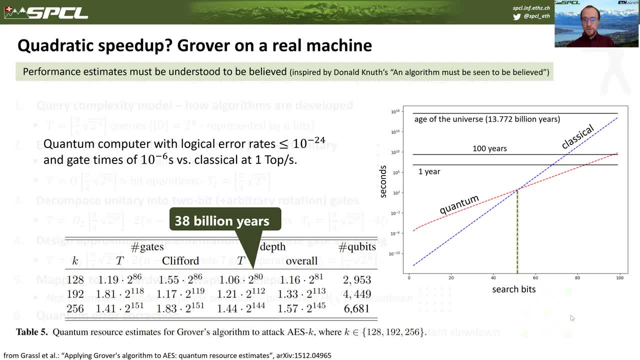 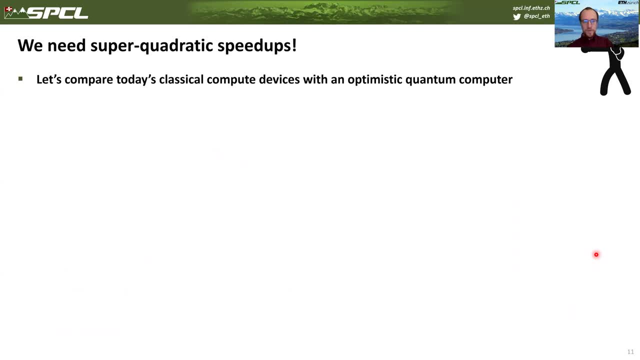 Asymmetric key schemes can be broken with Grover, so they're not super secure, but symmetric key schemes- at least I don't know that they're super vulnerable to this attack. So now, one last point I wanted to make is that actually Grover is not enough. 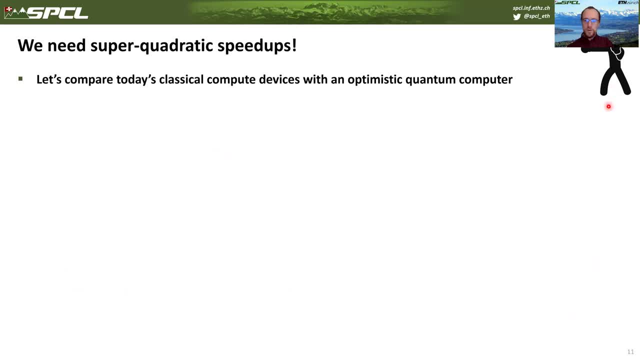 for pretty much any algorithm that you could imagine for near term quantum computers, because it only gives you quadratic speedup. So let us do a thought experiment: that we implement a classical computing device and we compare it with an optimistic quantum computer that I hope to see in the next 10 years. 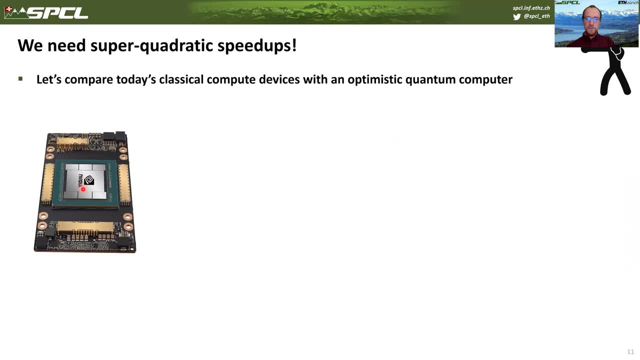 or maybe my lifetime. So our classical computing device is an A100, which we all know and love. So this A100 has about 10 terabit per second IO, 195 terabits per second FP16 bandwidth, nearly a hundred terabits in 32,. 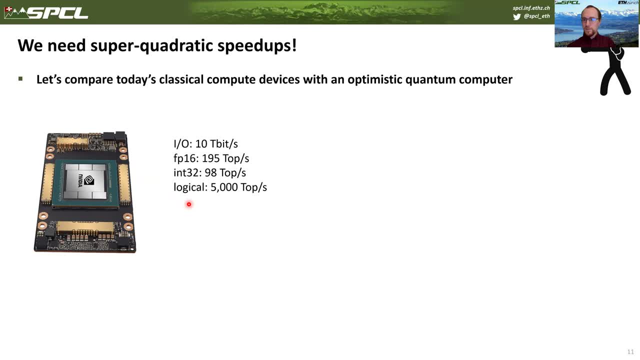 and 5,000 terabits logical, so binary operations at least. if we would implement it with the same chip technology, Then we have our lovely competitor, quantum computer here that has one gigabit per second IO. As I mentioned, it's quite hard to create quantum states. 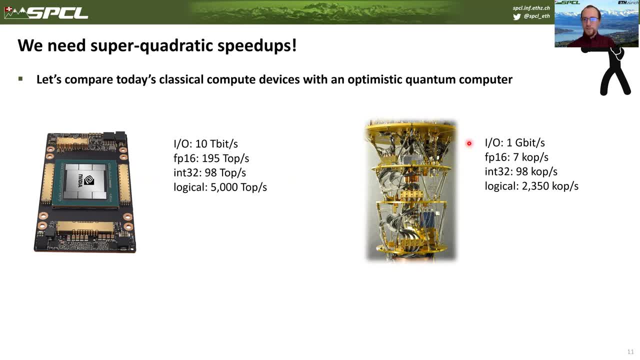 We do have another paper appearing at the Design Automation Conference this year on creating sparse quantum states, which is also not super simple. but this of course is: this computer, in addition to the IO limit also has a throughput limit. Like it can only do 7,000 operations or 98,000 operations. 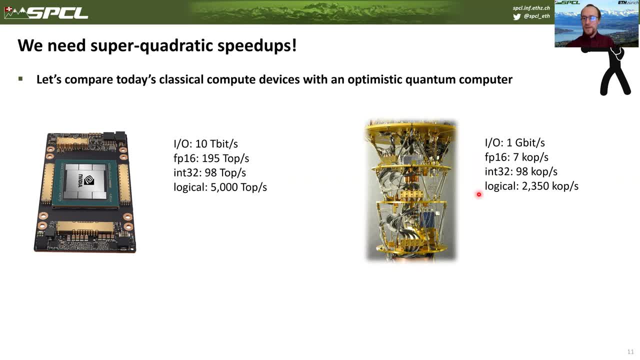 for FP16 in 32 respectively, And on the logical side it's also not extremely strong. So your A100 is now wondering: why am I even competing against this thing? Why are people investing millions of dollars They can just buy me for? I don't know. 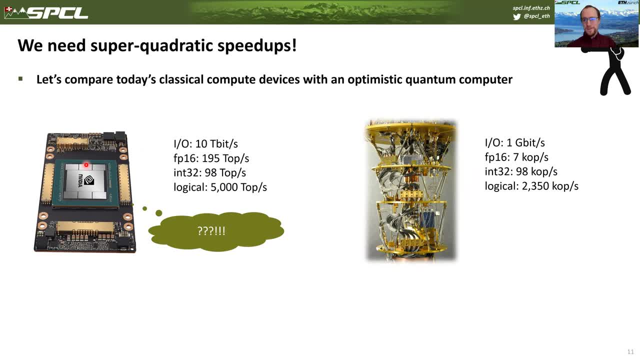 the cost of my car, I guess. So it's still not cheap, but it's also not millions of dollars. The quantum computer, as we just mentioned, only needs to evaluate the function square root n times. Well, this guy needs to evaluate it n times. essentially, 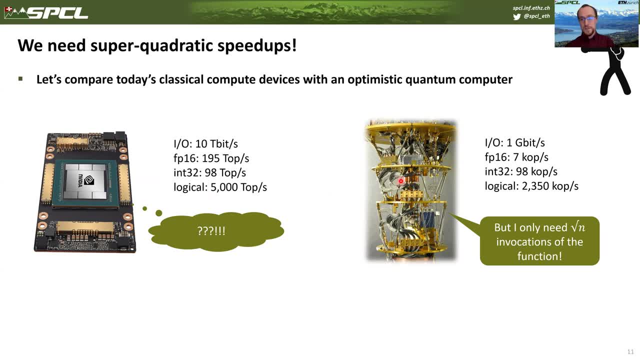 to implement the Grover algorithm or any quadratic speedup. So quite interesting speedup possibilities. So polynomial, not exponential, and this is just one algorithm that's the most versatile one. So now we assume a two-week runtime, like we allow these two computers to compete. 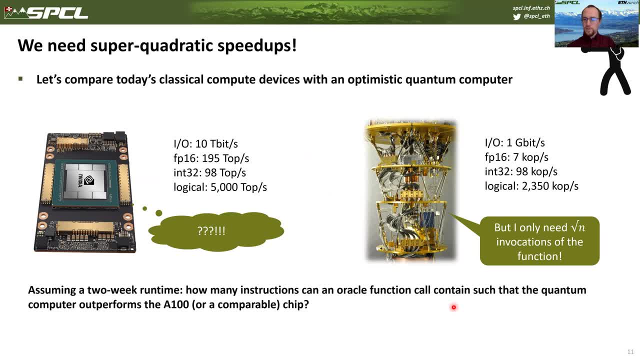 in a two-week time window? How many instructions can this oracle function contain such that the quantum computer actually outperforms the A100 or a comparable chip? That's a valid question. It's not super easy to answer if I give you just a result. 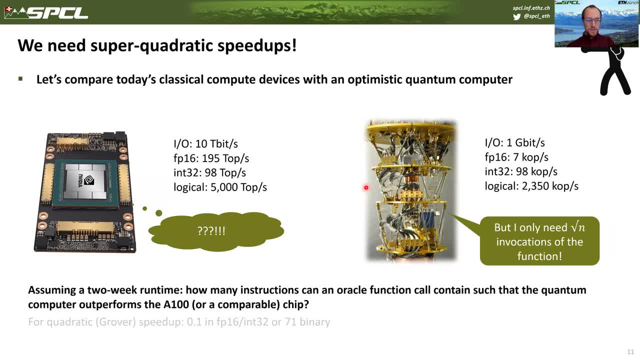 and we have a paper forthcoming on this that will appear as an opinion article. So for the quadratic Grover speedup, unfortunately only 0.1 operations, So not even a single FP16 or N32 operation could be included in my oracle or 71 binary. 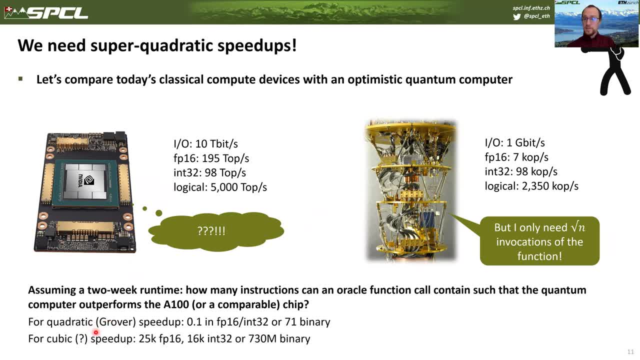 If we had cubic speedup, where we know no such algorithm, that is as generic as the Grover algorithm, we can have 25,000, 16,000, and so on, Or even 730 million. So much more realistic, but unfortunately we. 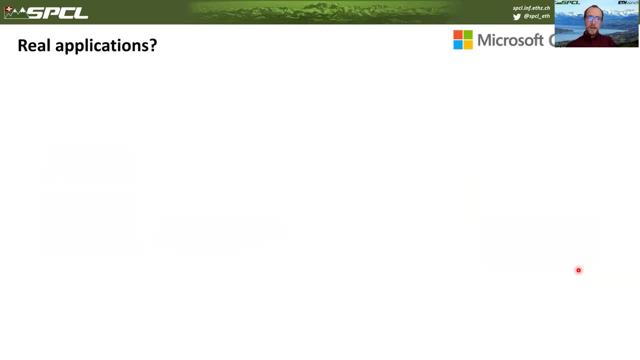 don't know a Grover-style algorithm, So I want to close my talk with an outlook towards real applications, towards nice applications that I'm really looking forward to, like quantum chemistry and quantum physics. It's the original idea by Feynman. 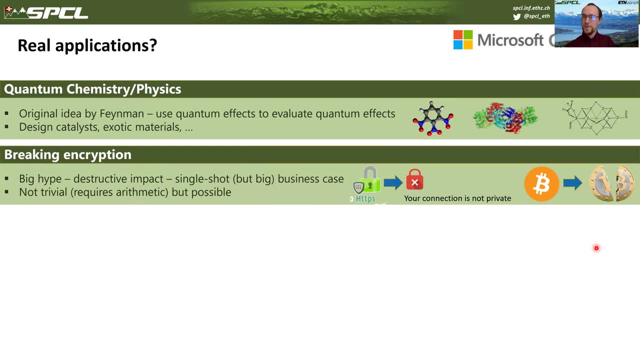 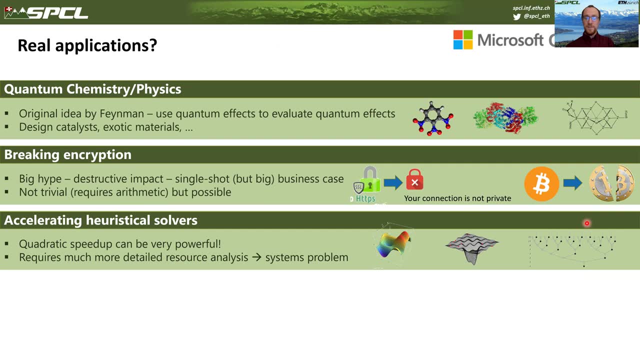 Breaking encryption. I'm not looking forward to this, but this will definitely happen, at least as a one-shot application And accelerating heuristical solvers where a quadratic speedup can be powerful. but it needs to have a very detailed resource analysis.